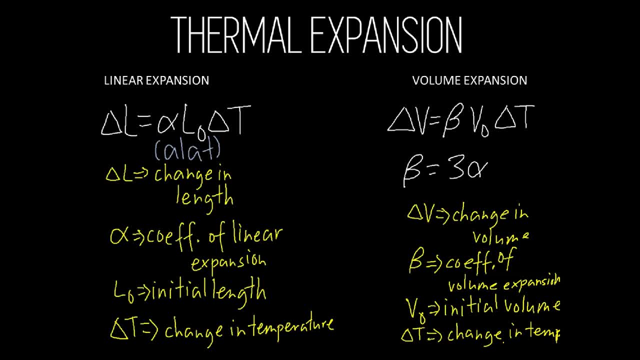 Delta V is equal to delta B, V naught times delta T. And beta is the thrice of the linear expansion coefficient. So the variable, The variables here for our volume expansion are the following: so it's the change in volume. delta V is the change in volume, V naught is the original length. delta T is the change in temperature. beta is the coefficient of volume expansion and, as I have said earlier, beta is thrice the linear expansion, so it is 3 times alpha. 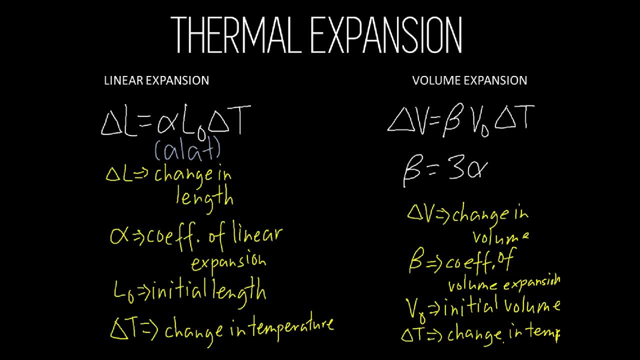 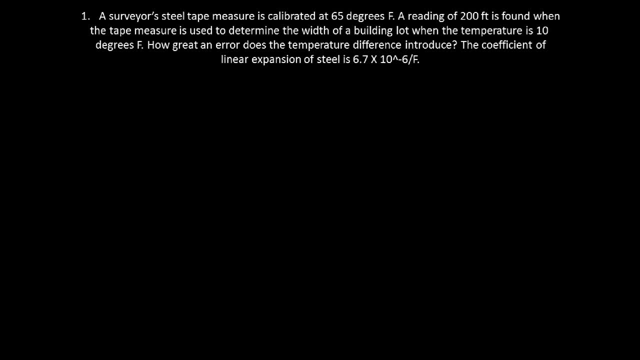 So now we're going to solve some problems involving thermal expansion. Okay, so let's read this problem. A surveyor's steel tape measure is calibrated at 65 degrees Fahrenheit. A reading of 200 feet is found when the temperature Temperature. 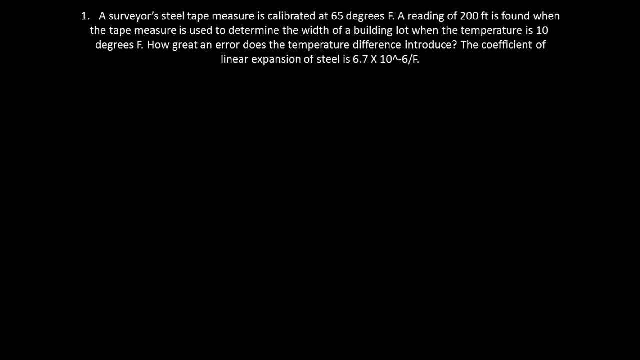 The tape measure is used to determine the width of a building lot when the temperature is 10 degrees Fahrenheit. How great an error does the temperature difference introduce? The coefficient of linear expansion of steel is 6.7 times 10, raised to negative 6 over degrees Fahrenheit. 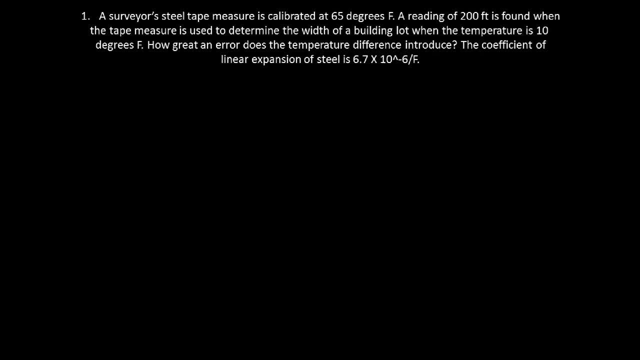 So what are the given values for this problem? So the given values Given Is the L naught, which is the original length. The original length of Over here is 200 feet. The alpha is also given. The alpha is our linear expansion coefficient. 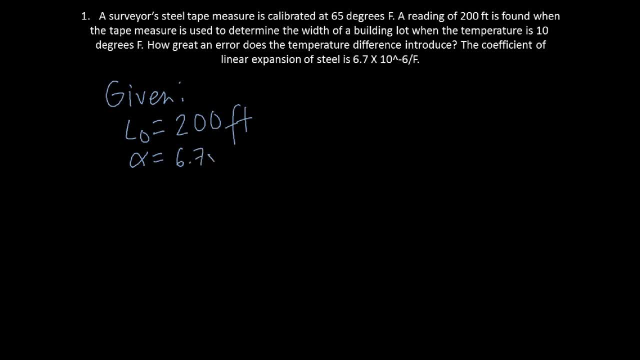 That is 6.7 times 10, raised to negative 6 over degrees Fahrenheit. So I'm just going to put degrees Fahrenheit. Now we're going to solve for delta T And then, Well, we know that That the final temperature is 65 degrees Fahrenheit. 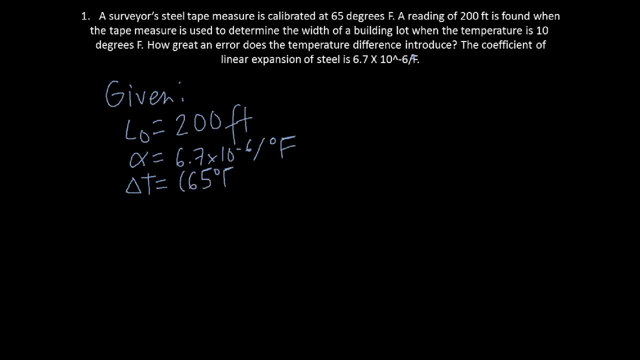 Okay, And the initial temperature is 10 degrees Fahrenheit, So our delta T will be equal to 55 degrees Fahrenheit. Now the required in our problem. what we need to find is the delta L. Okay, So the change in length. 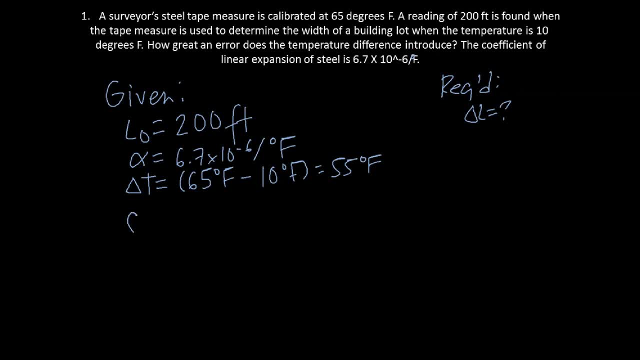 Okay, So the solution for this problem would be the simple formula that we use when we're finding for the change in length in our substance considered. So we remember the mnemonic, which is ALAT, So alpha times L, naught times delta T. 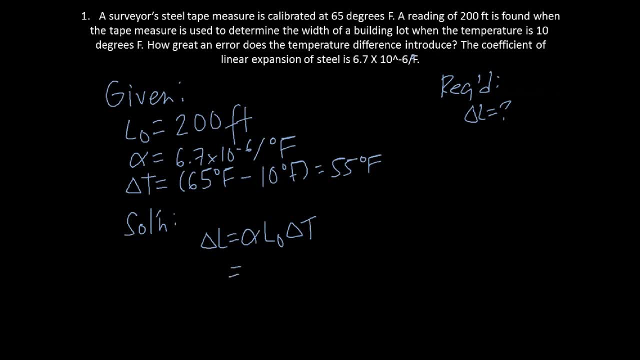 And then we have here Substitution of values. So 6.7 times 10, raised to negative, 6 times L, naught 200 times 55. And our final answer would be 0.0737 feet. Here is our final answer. 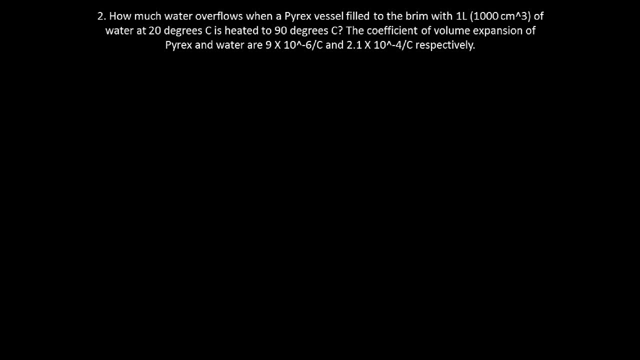 Okay, So this would be our last problem for this video. So let's read and pause the video if we're going to solve it. So how much water overflows when a Pyrex vessel filled to the brim with 1 liter or 1,000 cubic centimeter of water at 20 degrees Celsius is heated to 90 degrees Celsius? 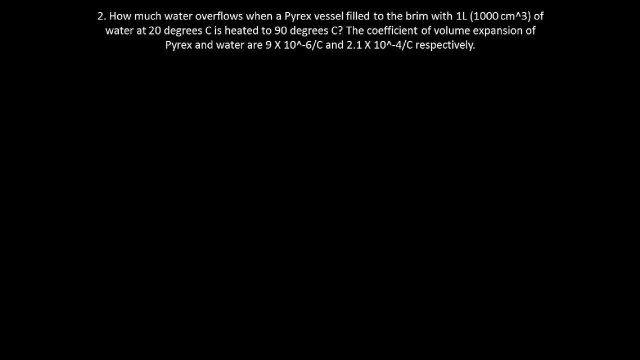 The coefficient of volume expansion of Pyrex and water are 9 times 10 raised to negative 6 over the Degrees Celsius, And 2.1 times 10 raised to negative 4, divided by degrees Celsius respectively. So we're going to list the given and the required. 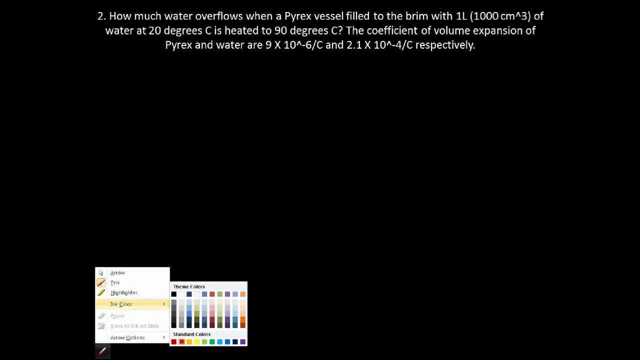 So, and then the ink color should be light Right there, Okay. So the given values for this problem are the following: So V naught Is equal to 1 liter or 1,000 cubic centimeter, And then our delta T will be, of course, final temperature minus the initial temperature. 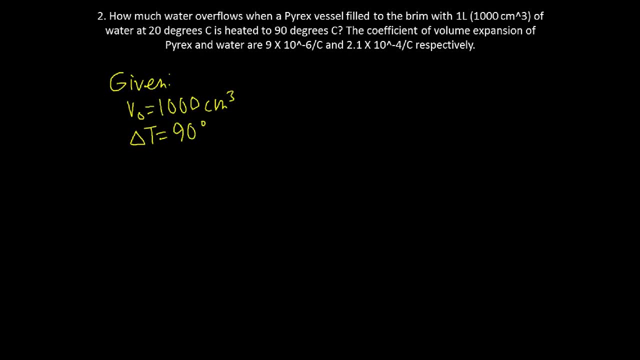 So 90 degrees Celsius minus 20 degrees Celsius is equal to 70 degrees Celsius. And then the beta, or the volume expansion coefficient of water, Okay, Is equal to 210 times 10 raised to negative 6, divided by degrees Celsius. 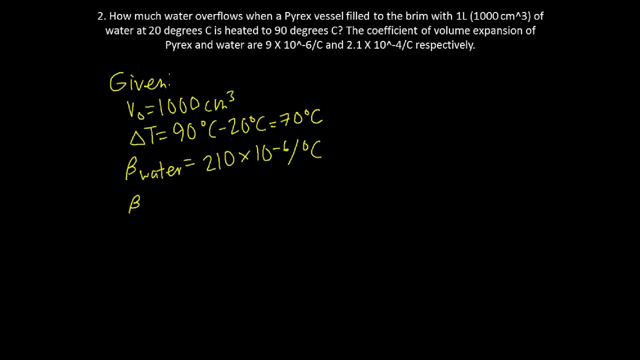 And then, finally, the volume expansion coefficient of Pyrex is equal to 9 times 10, raised to negative 6 degrees Celsius. What we are required to find here Is, of course, the water that overflowed from the Pyrex vessel. 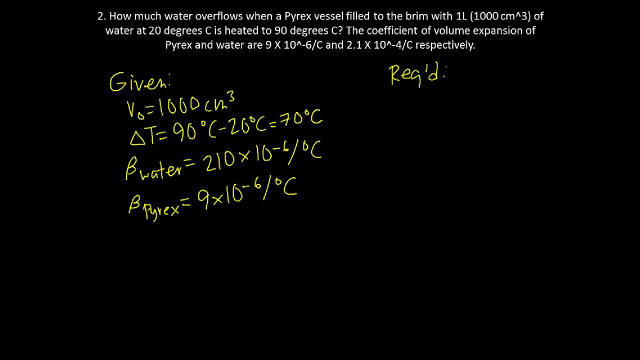 So how do we find that? So it is the volume overflow, And our volume overflow will be equal to the volume of water that surpassed the volume of the Pyrex. So we're going to subtract that, Subtract that with the volume of the Pyrex vessel. 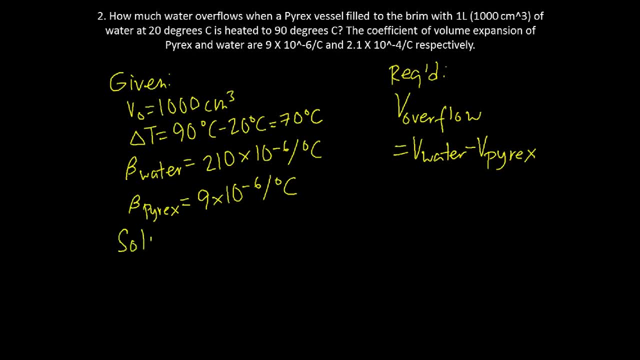 So here's our solution to this problem. So V overflow is equal to V water minus V Pyrex. So it will be: V overflow equals V sub water, So V sub water will be when we're going to expand the formula. 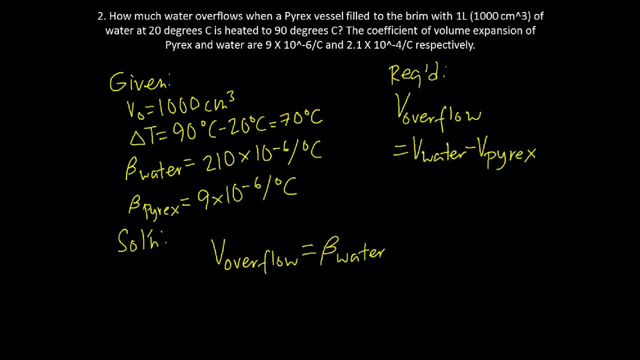 Delta water times. V naught Times delta T minus the volume expansion of the Pyrex, And then the same variables. Now we're going to factor out the common variables, The common variables, that is, the V naught times delta T. 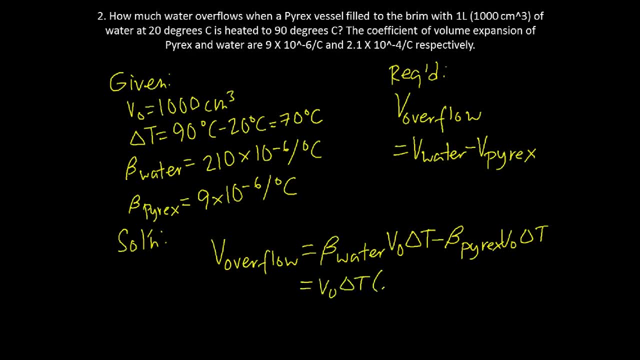 So V naught delta T Factor that out Beta water minus beta Pyrex. Okay, So we're going to supply the variables. So 1,000. Times 1,000 times delta T will be 70 degrees Celsius. 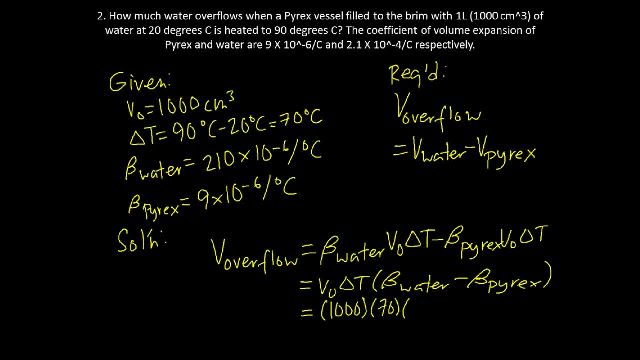 And then the beta water: 210 times 10 raised to negative 6.. Minus beta Pyrex will be 9 times 10 raised to negative 6.. And then our final answer will be 14.8.. 1 cubic centimeter.